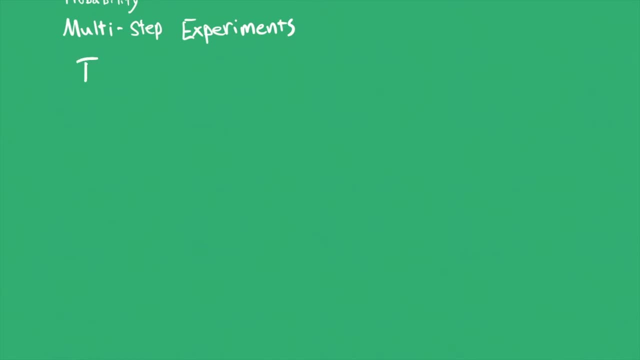 One way to do this is by drawing a tree diagram. A tree diagram is the most useful way to represent graphically multi-step experiments. Let's start with a tree diagram. Let's look at the example of flipping two coins. For the first coin, there will be two results. It's either head or tail. 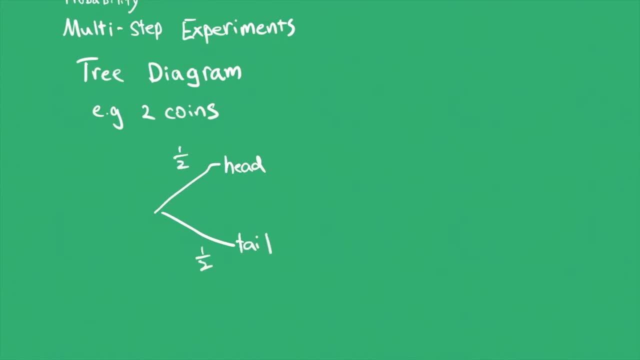 and each, the chance would be half. If we go ahead for the first flip, we'll need to do the second flip, which brings us the same result head and tail, and the probability of it would be the same same as the tail one. 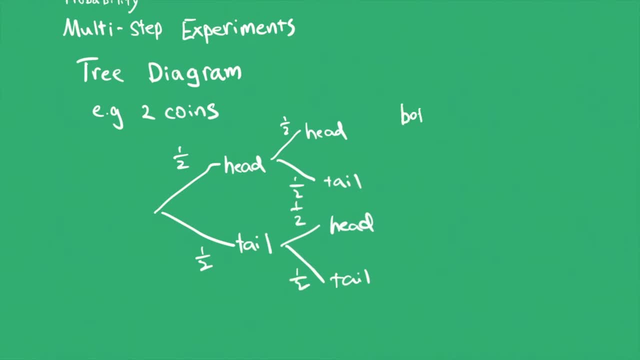 And if we want to find the chance that both flip would be head, we just need to times the first probability by the second. In this case, half times half would be a quarter. So a quarter would be the probability of getting two heads. 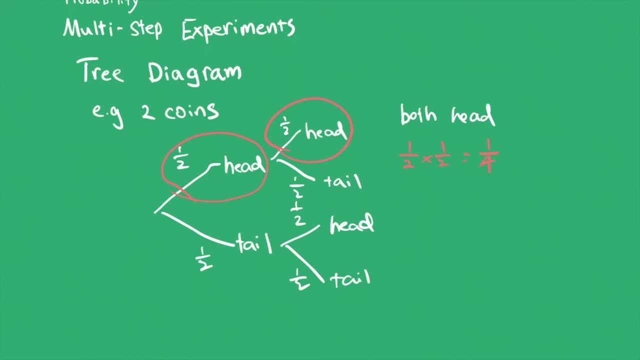 This can also be shown through the conditional probability formula in this case. And if we want to find multiple probabilities- in this case, let's say both tail and both head- we just need to add the two heads. And if we want to find multiple probabilities- in this case, let's say both tail and both head- we just need to add the two heads. And if we want to find multiple probabilities- in this case, let's say both tail and both head- we just need to add the two heads. And if we want to find multiple probabilities- in this case, let's say both tail and both head- we just need to add the two heads. 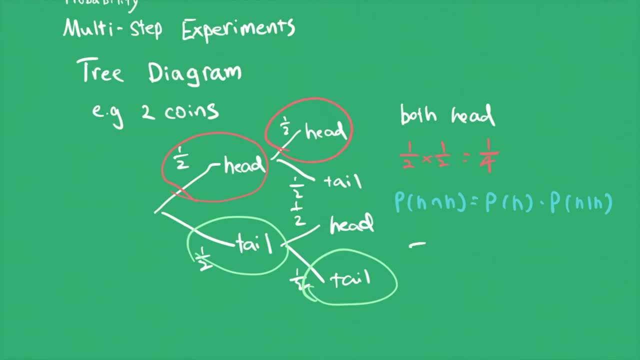 We need to find multiple probabilities of each one together. in this case, half times half plus half times half equals to a half, So a half would be the probability of both head and both tail. Okay, now let me show you an example. question: 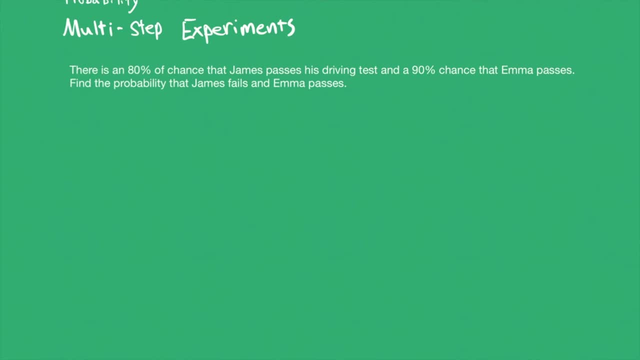 There is an 80% chance that James passes his driving test and a 90% chance that Emma passes hers. Find the probability that James fails and Emma passes. To do this question, we can first draw a tree diagram. Let's show James' probability first, The probability that James passes his driving.